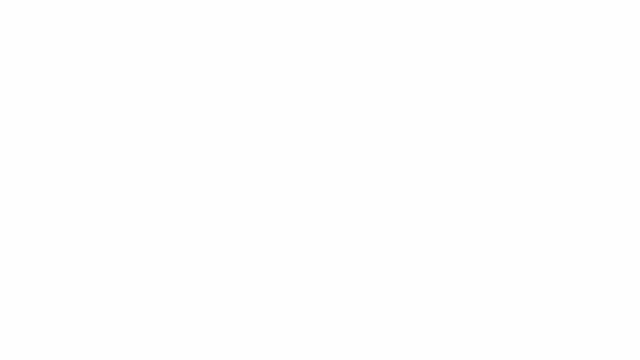 How do we find the inverse of matrix A here? It's a 3 by 3 matrix this time. The formula for A inverse that we saw in the previous lesson is valid for all square matrices. It's equal to 1 over the determinant of A multiplied by the adjoint of A. 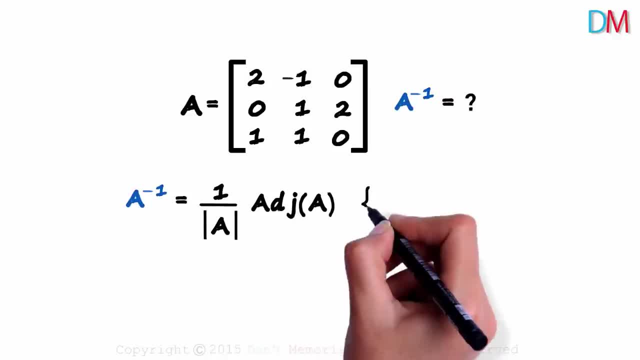 No elementary operations needed. The condition states that the determinant of A must not be equal to zero. That's because the denominator cannot be equal to zero. If the determinant of A is zero, then we can say that the inverse of matrix A does not. 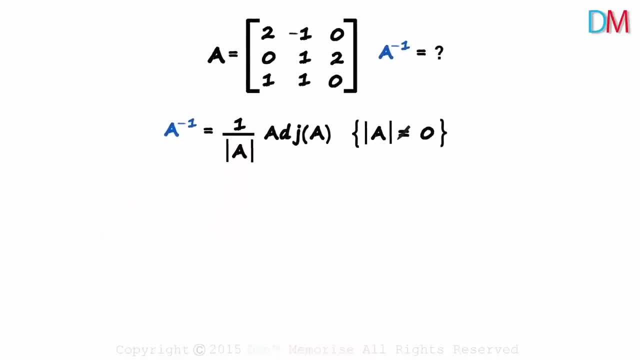 exist. So that's the first thing we should do. We find the determinant of A. We can have the first row as the reference, Because we've already solved innumerable determinant problems. let's go through this quickly. The element two will be multiplied with this determinant to get this. 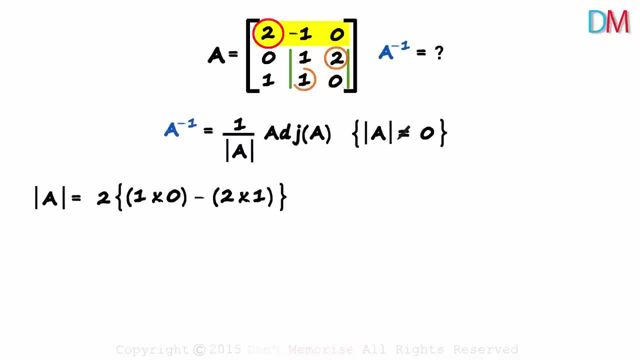 Two multiplied with one times zero, minus two times one. The next element is minus one. We get this Minus because we are multiplying this product with minus one raised to one plus two. The last element for the first row is zero. Because it's zero, it doesn't matter what it's multiplied with. 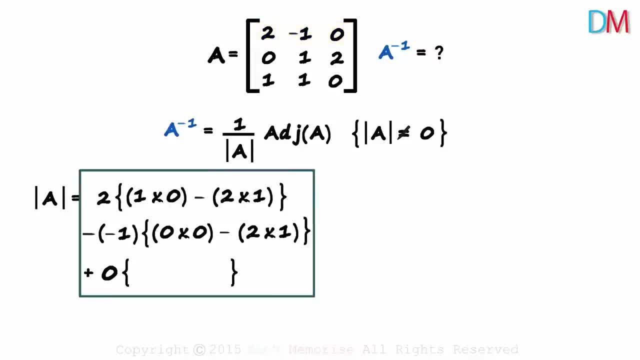 The product will always be zero. This will be the value of the determinant. This part in the brackets will equal zero minus two, which equals minus two. Two times minus two will equal minus four. What about the second product Inside the brackets? we have zero minus two, which equals minus two. 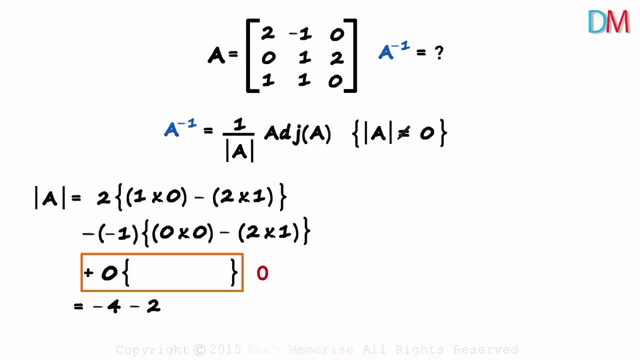 One times minus two is minus two And this product is zero. Minus four minus two will equal minus six. We have the determinant now. It's minus six, It's minus six, It's not equal to zero. We can say that it's non-singular. 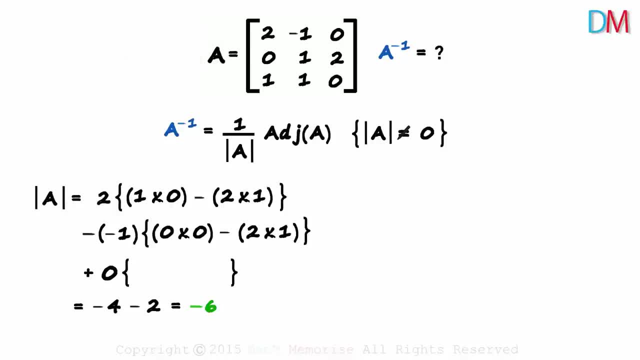 The inverse of this matrix exists. So we can move on to finding the adjoint of A now. To find the adjoint, we first find the matrix of cofactors of each of the elements and then find the transpose of that matrix. So let's find the cofactors of each of the elements now. 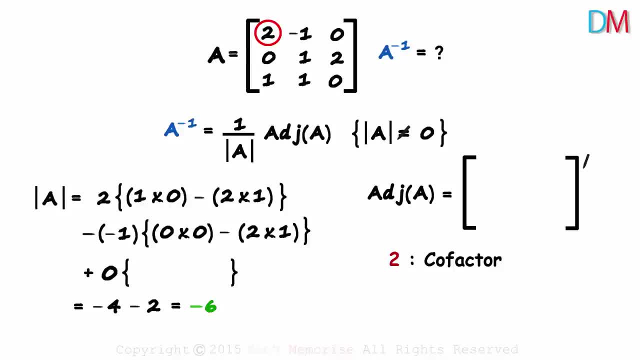 The first element is two. Its cofactor will equal minus one raised to one, plus one times its minor. Its minor is the determinant of what's left after excluding its row and column. So the cofactor will equal one multiplied by zero. minus two, minus two. 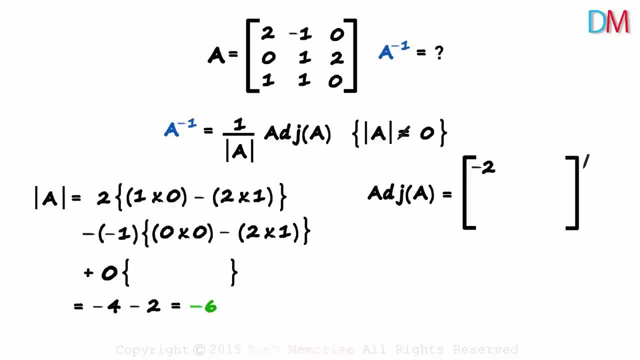 The cofactor of this two is minus two. Now we come to the cofactor of minus one. It will equal minus one raised to one plus two times zero times zero, minus two times one. Minus one times minus two is two. Minus one times minus two is two. 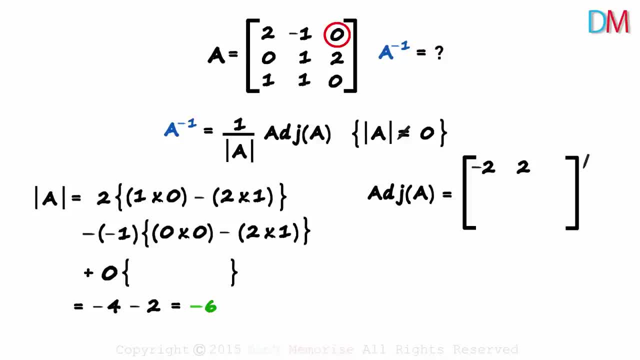 Minus one times minus two is two. Similarly, we get the cofactor of zero as minus one. Now please pause the video, take your time and solve for the remaining six cofactors. These are the six remaining cofactors. This transpose will give us the adjoint of matrix A. 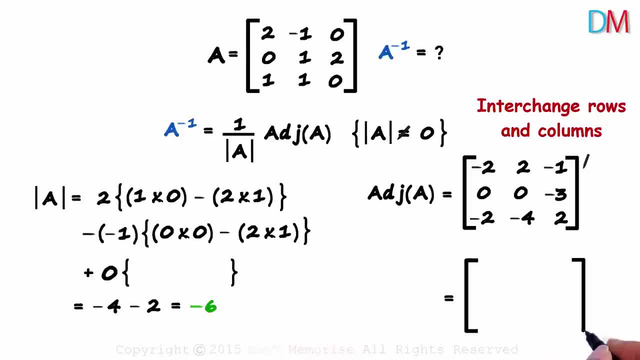 To find the transpose, we interchange the rows and the columns. The first row will become the first column, Two minus one. The second row will be the second column: Zero, zero minus three And, lastly, the third row will become the third column. 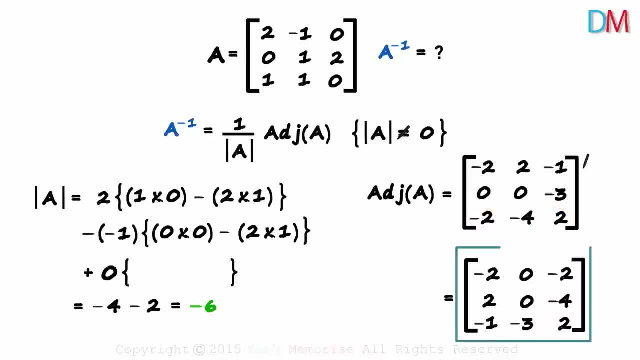 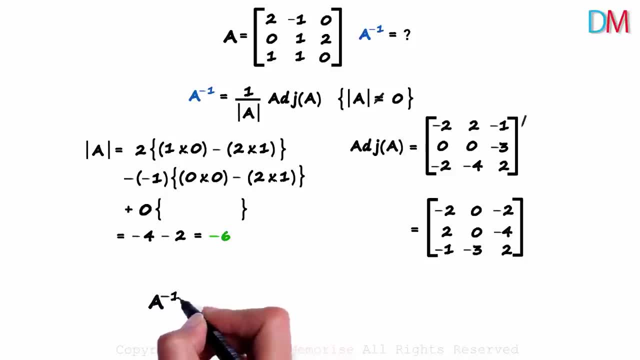 Minus two minus four two. Now we have the adjoint as well, And because we have both, we can find A inverse. now Let's write it here: One over determinant of A will be one over minus six. We multiply this with the adjoint of A. 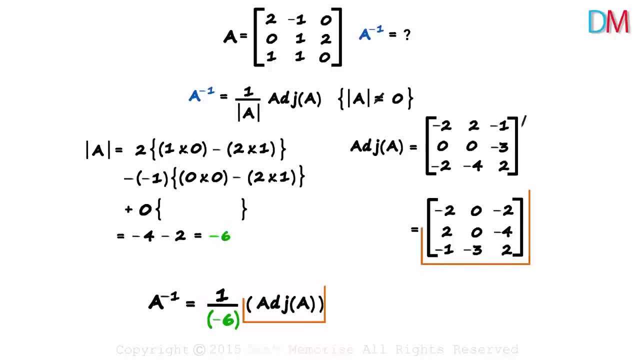 What is this? What will this be equal to? This is the adjoint. To get this, we multiply this scalar with each element of the adjoint. One over minus six times minus two will equal one over three. One over minus six times zero will equal zero. 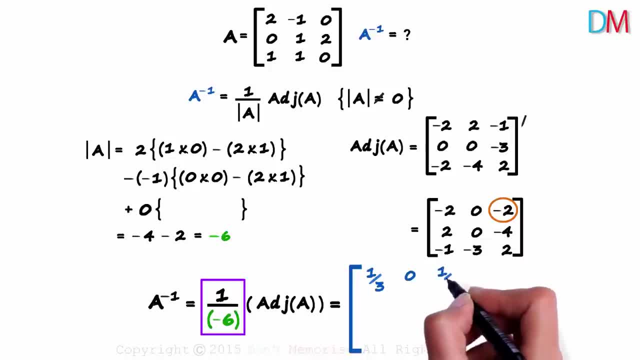 One over minus six times minus two will equal one over three again, And, like always, I want you to find the remaining six elements. Remember We need to multiply each of the elements. Remember We need to find the remaining six elements with this scalar.